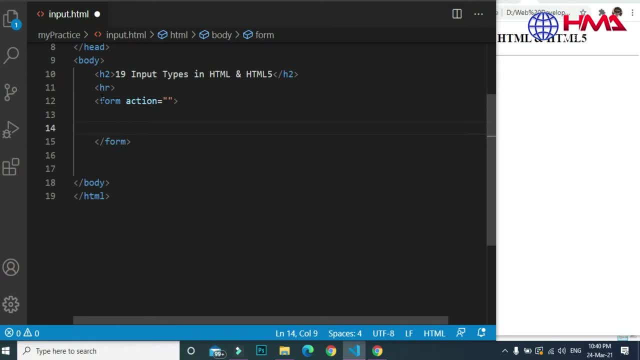 First of all, let's start creating an HTML form tag And inside the form tag, we are going to create our input fields, which will be included in our form. First of all, we have to write the label tag. Label tag is used to describe the input field. 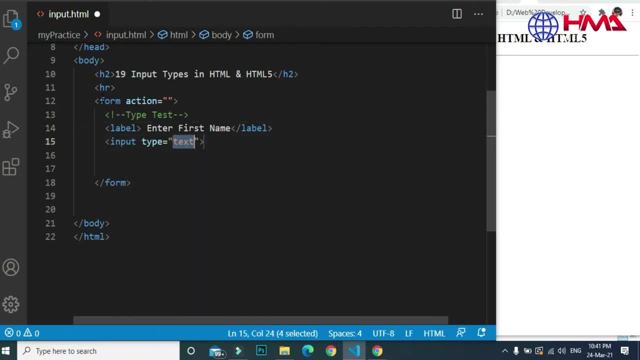 First input is enter first name. The type of this input is text And name of the input is first name. Placeholder is first name. Placeholder is just a faded text which will be displayed inside the input field To separate the each input in our form And our second input type is input type password. Let's copy paste all the above input And let's change this. 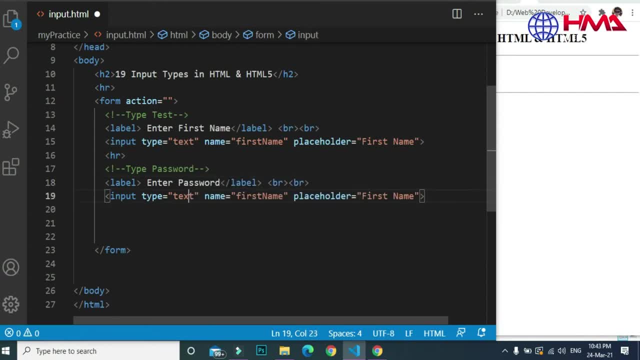 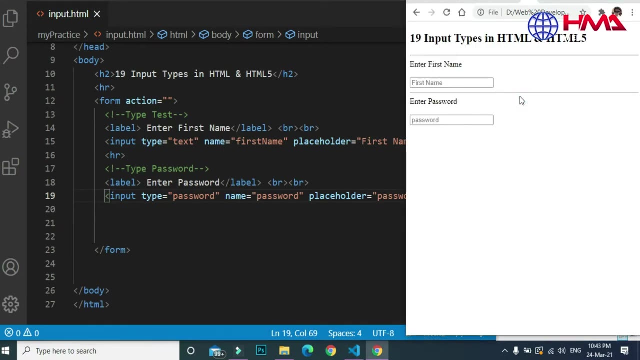 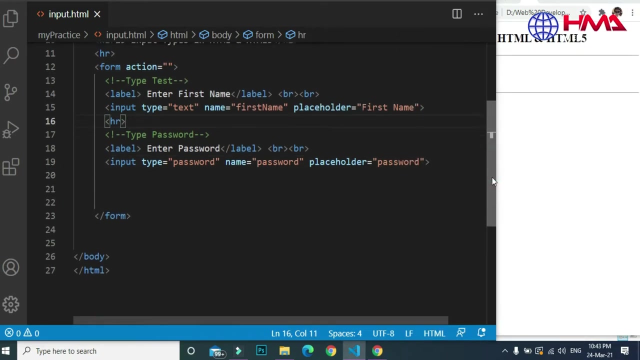 Enter password. Type of this input is password. This input will allow user to enter password, And password will not be displayed to the user. And this is the output. This is, we can enter password. Now let's move further. Our next input type is: 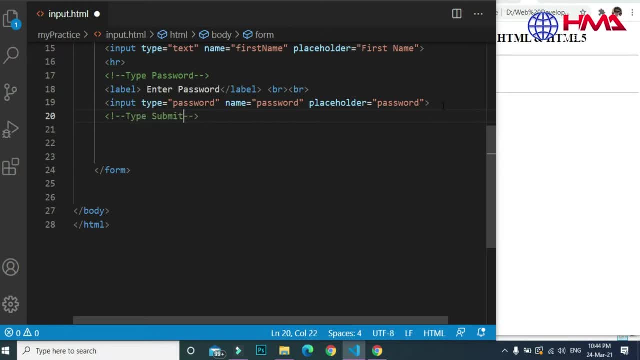 Input type: submit- HR. for the horizontal line. Let's copy and paste the previous code And we are changing this code. This input type is submit. Name of the input is submit And value of the submit. This will create a submit button. 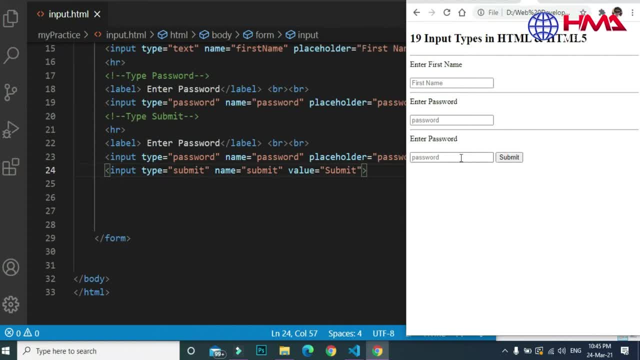 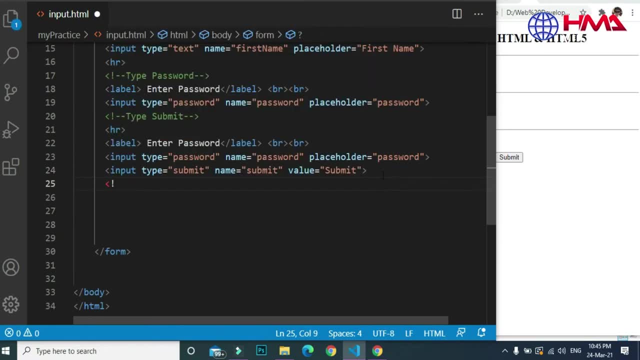 Which will be used to submit the form. Our next input type is type reset. This will create a reset button in our HTML form Which will be reset all of the input field Which have been filled earlier. This input type is reset. Value of this input is reset. 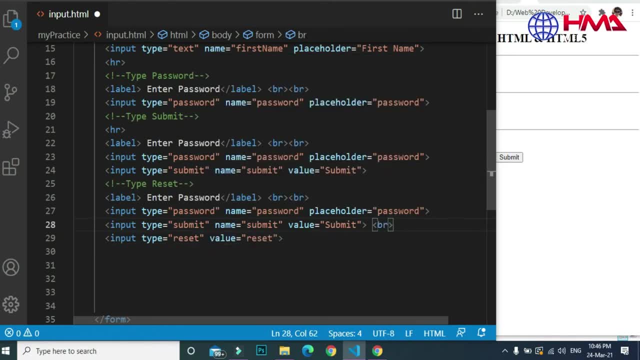 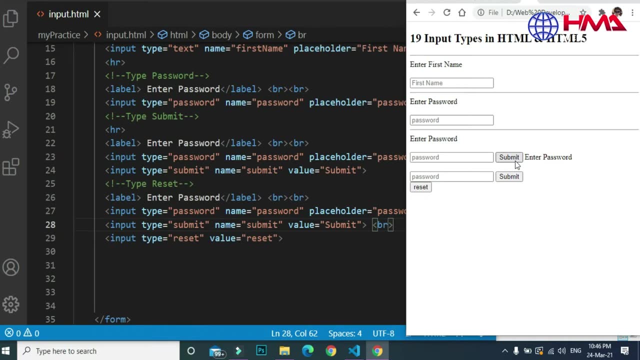 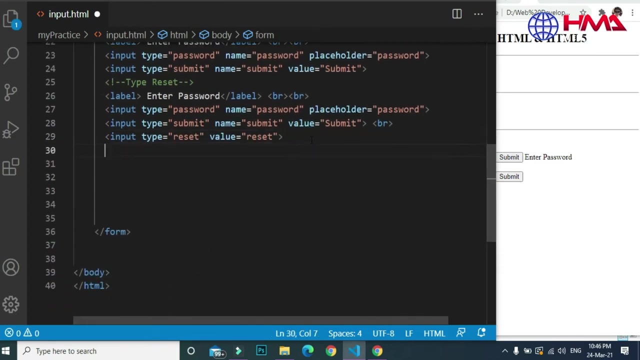 This will create a reset button in our form. So here is it. Let's type any password And press a reset button. Then password will be reset. Now our next input type is type radio. Let's create a label tag. What's your favorite color? 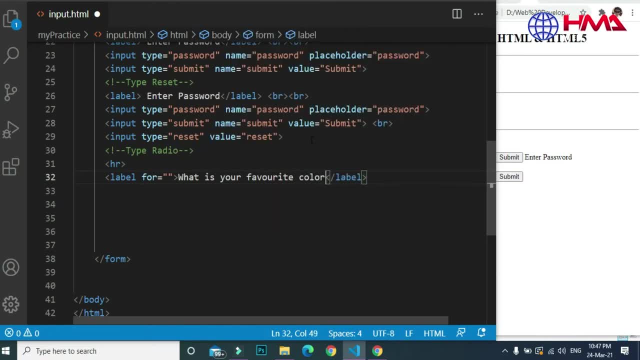 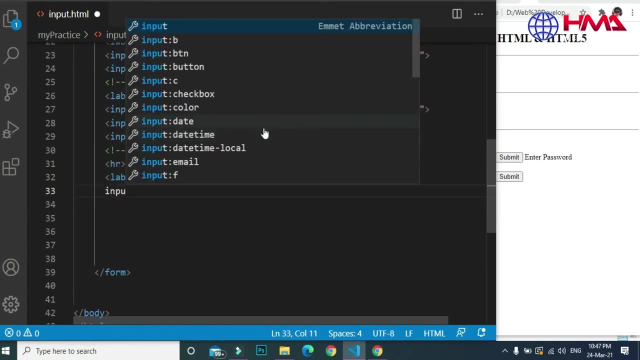 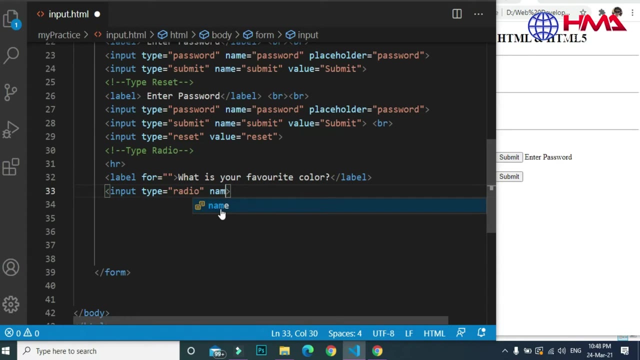 This is very important input type in HTML forms. This input type will allow user To select only one input from main inputs. Input type is radio And name of the input is color. First value is red. Second value is green. Let's create a third value. 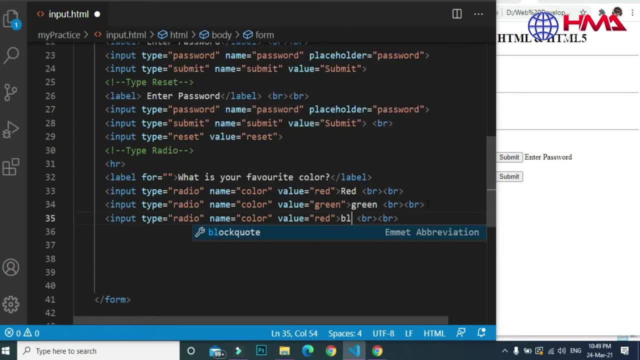 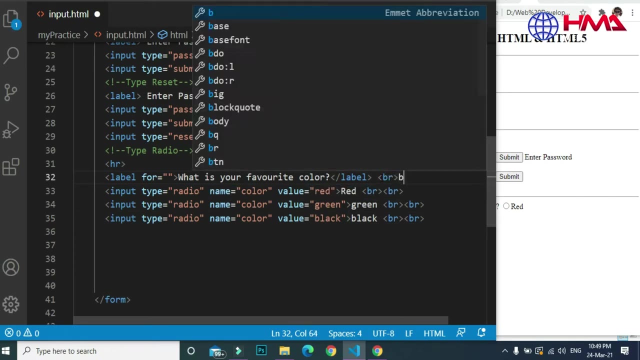 Which is black, And name of the input should be same, Which is color And value of this input will be different. This input will allow user To select only one option Out of many given options. Out of multiple options, User can select only one option. 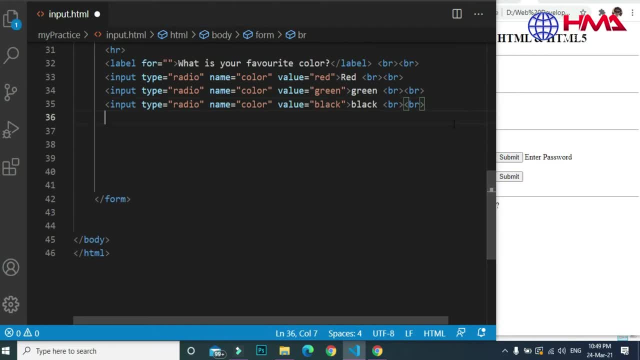 Now let's move further. Next input type is checkbox. This type is very similar to radio type, But the difference is that In this input User can select more than one option, So here The name of the input will be different. 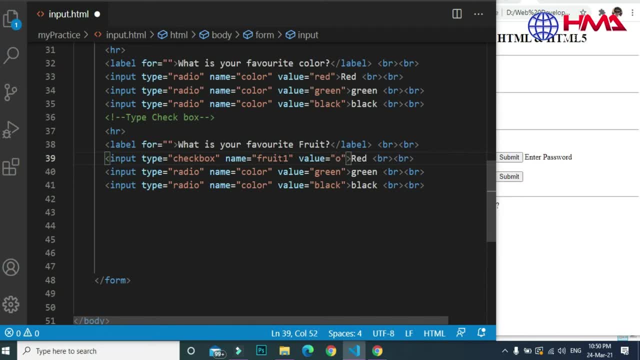 In the previous input, Radio type, We have written The name of the input same And in this input type Name of the input is different, Which will Allow user to select Their favorite. fruit Type is checkbox. Input name is fruit2.. 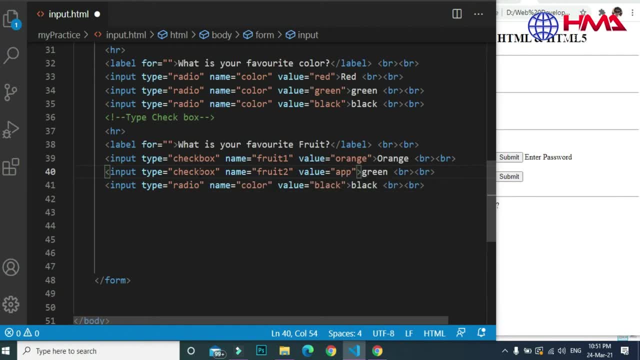 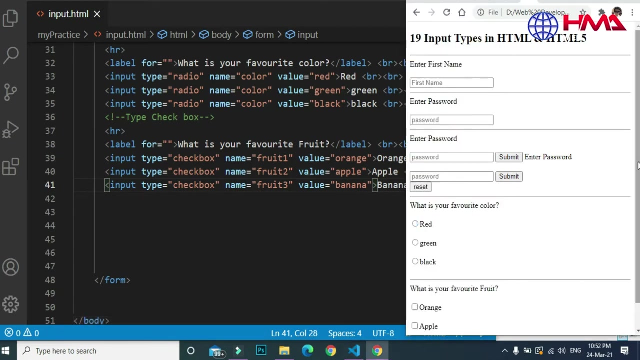 Fruit2. Is apple. Let's change third input: Banana. Value of this input is Banana And name of this input is Fruit3.. Name of all this input will be different Because user can select Multiple option in this input. 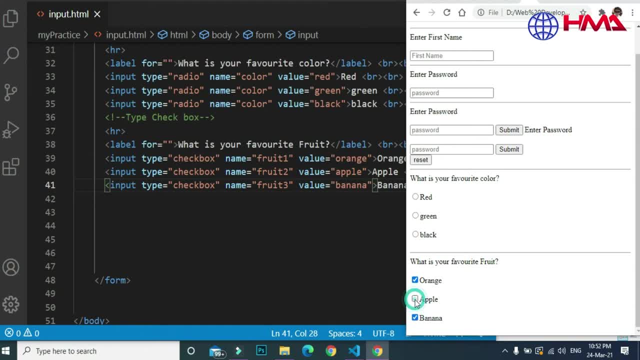 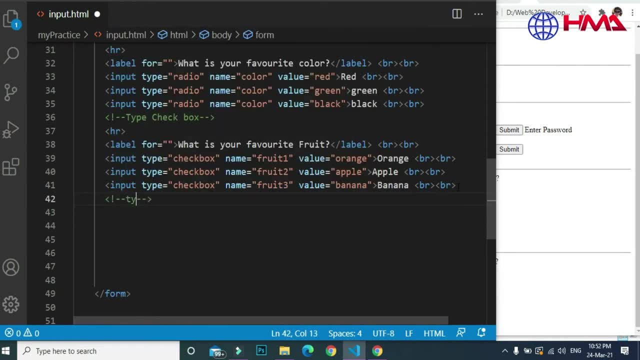 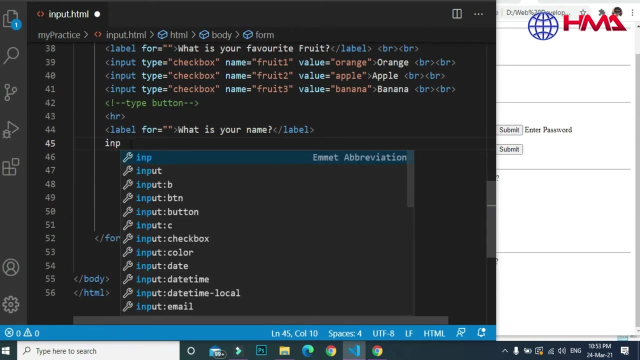 As we can see here, We can select all option As we want. Next, move further. The next input is Input type button. Let's write label tag. What is your name? Let's create Input tag And input tag in HTML. 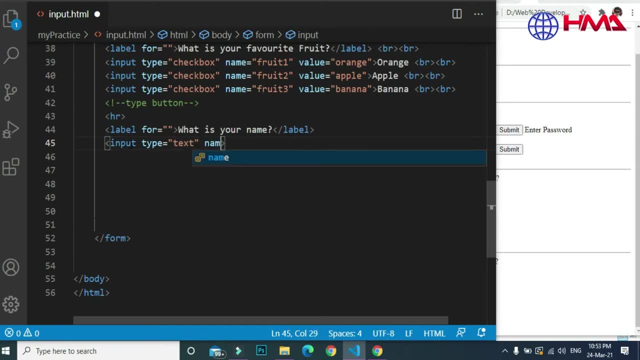 Don't have an end tag, It is only A single tag. input Type: text: name of the input name. Now next, input type button And value of the input is Submit. This input will also create A submit button Which will be used. 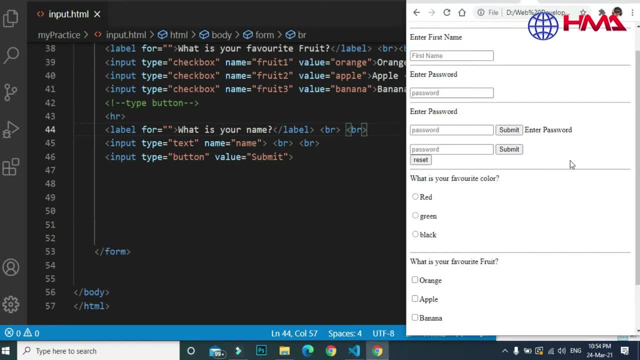 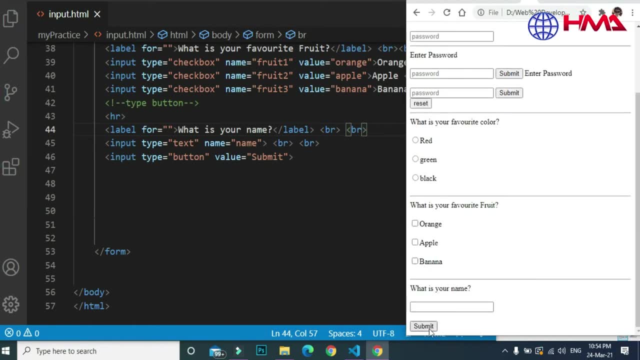 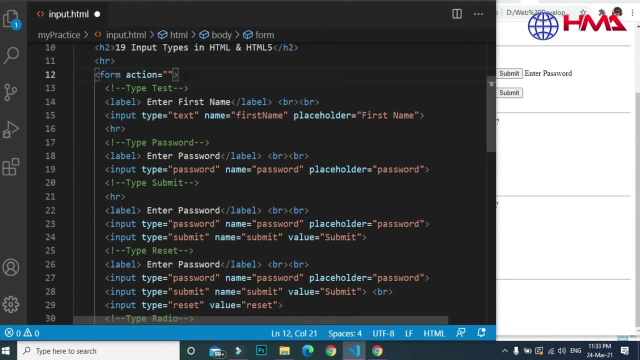 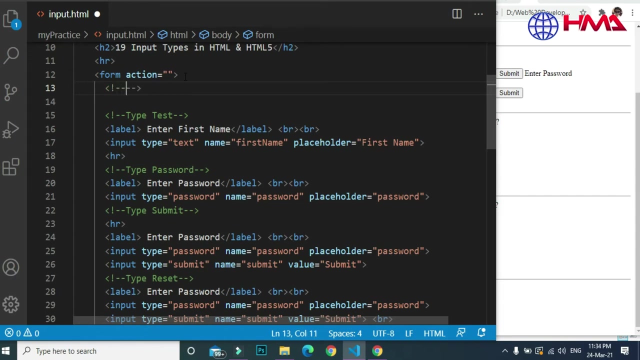 To submit the form data To the web server. Here is our input. We can submit The name Using The Submit button. Next, Right here We are going to write The next input type. Next type is Input type file. 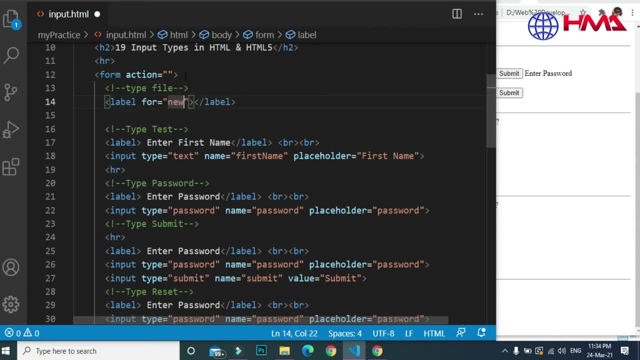 The file input in HTML Is very important, Which will Allow user To select And submit Any file From the computer Label for our computer Input is file. Select a file To upload. Input type Is file. 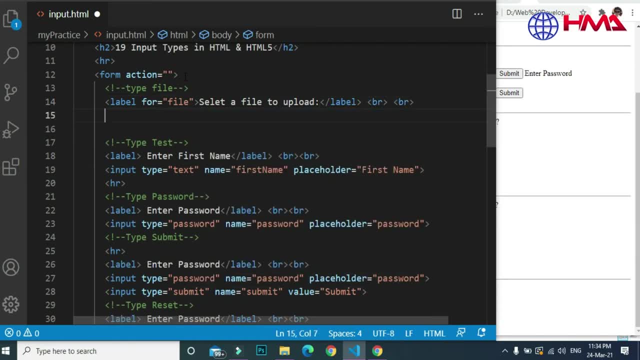 Name of the input Is file, ID is File And this ID Should Match To the For And Name Of The File And To the For Attribute In the Label tag. 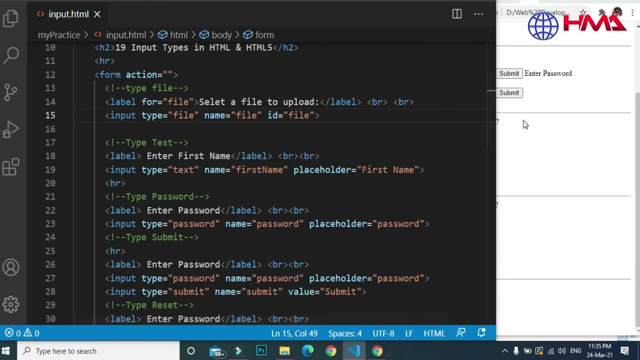 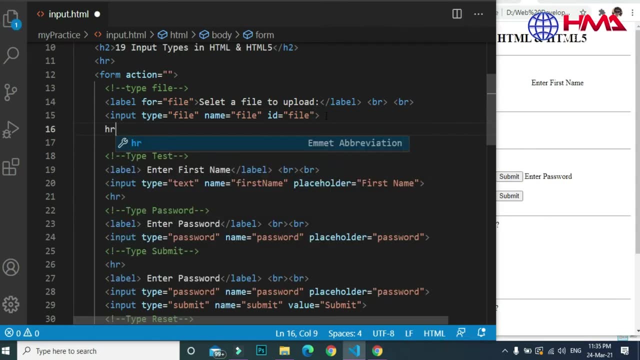 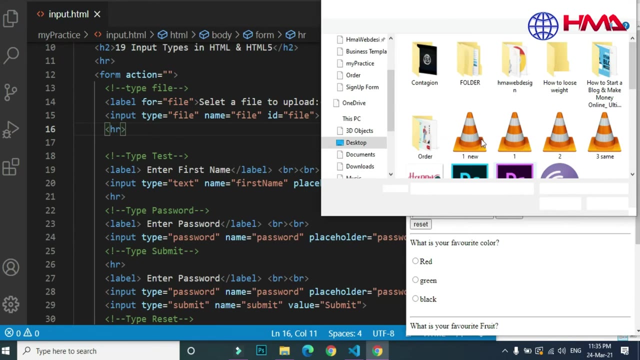 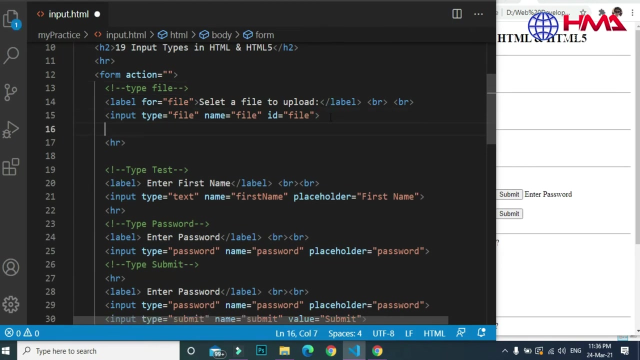 ID Attribute Will Be Similar To the For Attribute. User Can Select Here Only Single File. If We Want To Select Multiple File From Our Computer. 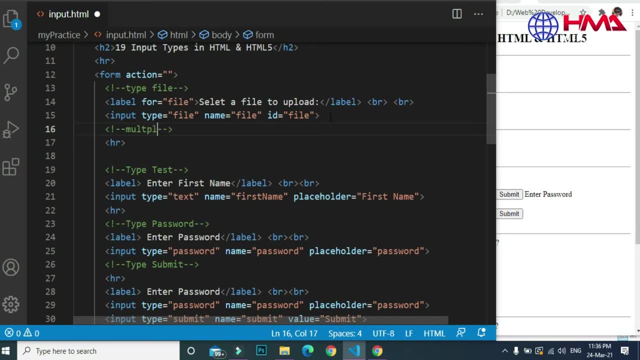 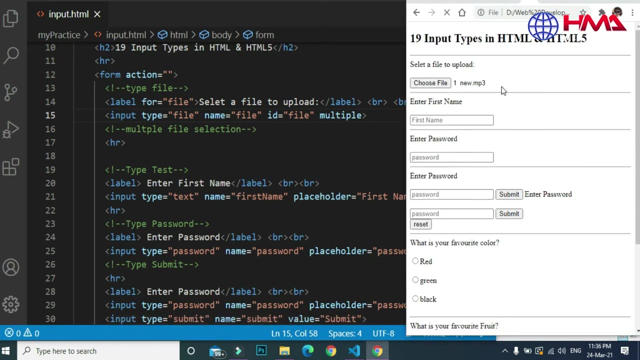 So We Have To Change Our Input With The Attribute Like Multiple. This Multiple Attribute Will Allow Us To Select Multiple File From Our Computer Now. 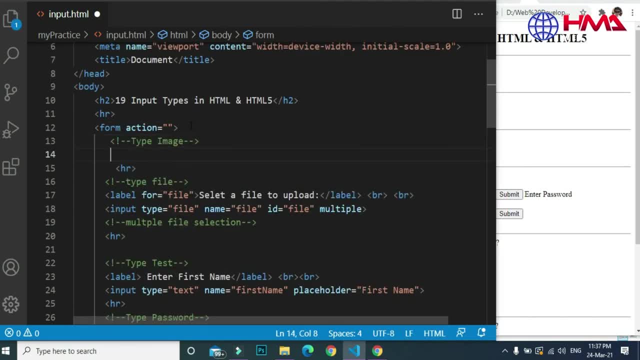 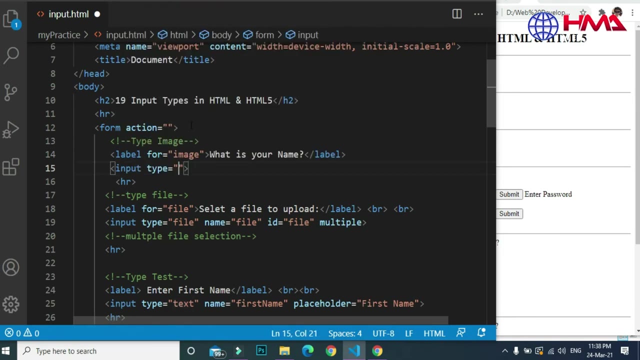 We Can Select More Image. What Is Your Name? We Can Also Make Image Input. We Can Also Use Any Image Input When User Click Click. 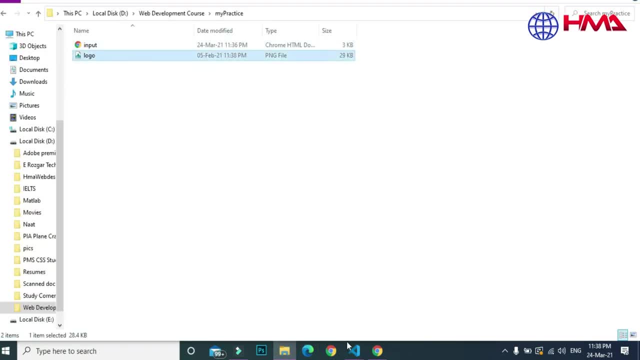 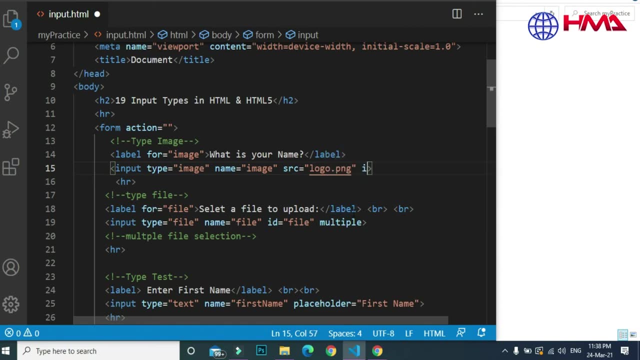 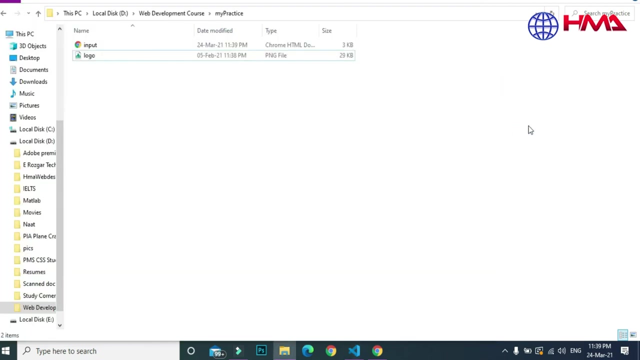 On This Image, Then Data Will Be. This Is The Image Name And Id Of This Input Is Image. Now User Can Submit The Form Data. 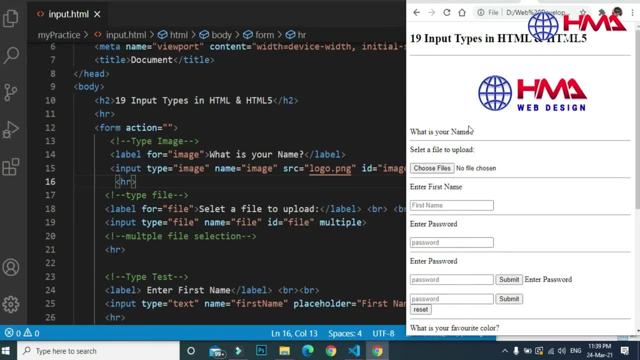 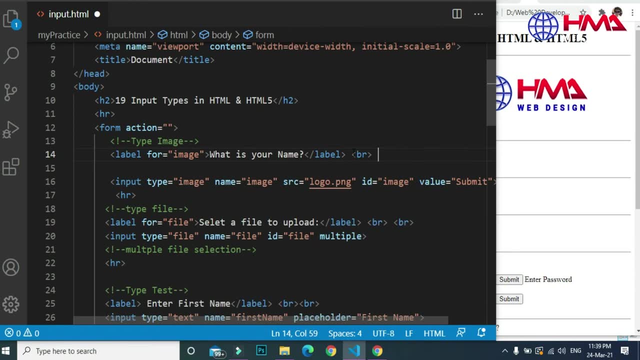 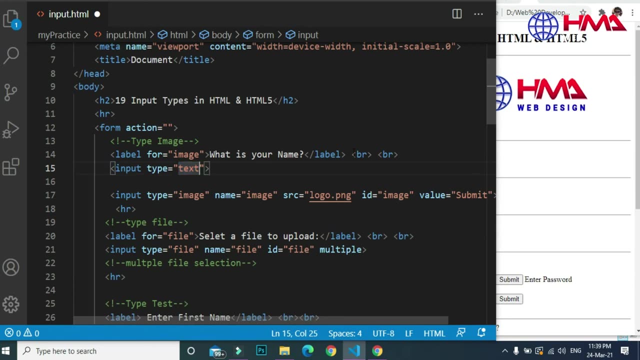 By Clicking On This Image, Let's Refresh Our Page. This A Couple Of Line Breaks To Display The Input In Separate Line. Here We